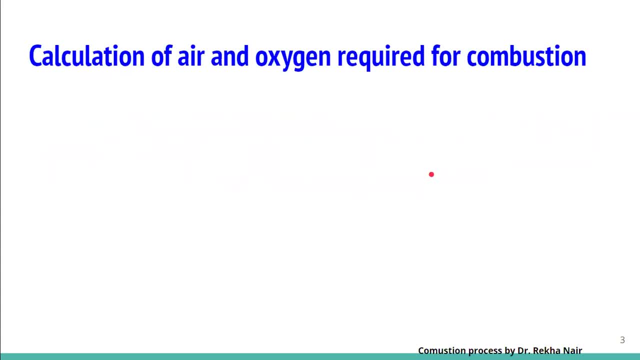 it is a reaction with oxygen and it releases some amount of energy. Now let us calculate the air and oxygen required for the compression process. Before going for the calculation, we must know some of the elementary principles applied for the calculation of oxygen and air. The first principle that is applied for the calculation is: air contains 21.4% of oxygen. 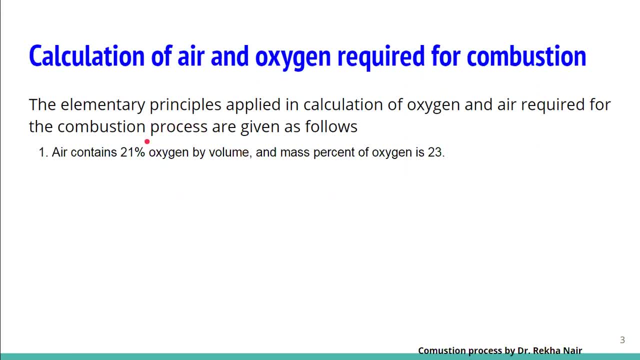 oxygen by volume. or else we can say that we assume that air contains only oxygen and nitrogen and all other elements are negligible. so if there is 21 percent of oxygen and the left out 79 percent is nothing but assumed as nitrogen. similarly, impose mass percentage of oxygen is 23, it means that there is 23. 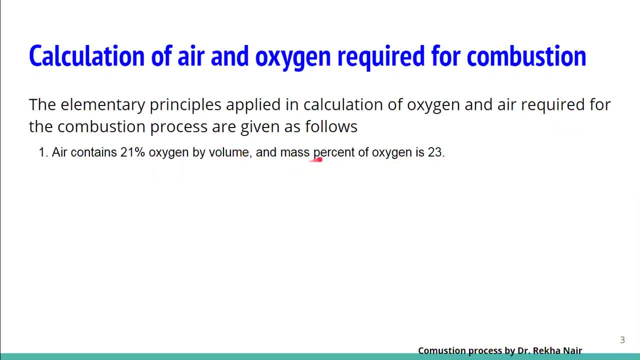 percent of oxygen in air in terms of mass percentage, and the remaining 77 percent is nothing but nitrogen. so the first assumption is: by volume, the air contains 21 percent of oxygen and in terms of mass it contains 23 percent. so if we want to calculate the amount of air, so 1 kg of 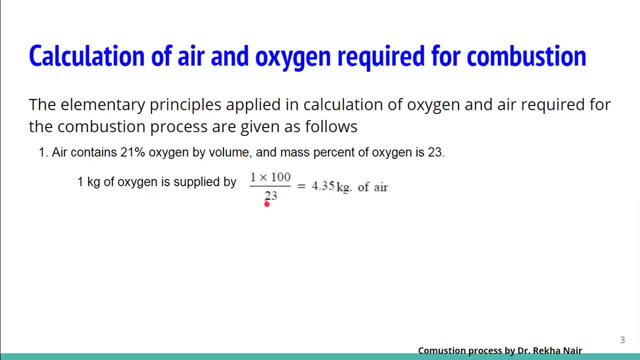 oxygen is supplied by 1 into hundred upon 23, that is 4.35 kg of air, whereas 1 meter cube of oxygen is supplied by 1 into 100 upon 21, that is 4.76 meter cube of air. In terms of mass, we are multiplying it with 100 upon 23 and in terms of volume, it is multiplied by 100 upon 21 to get the amount of air. 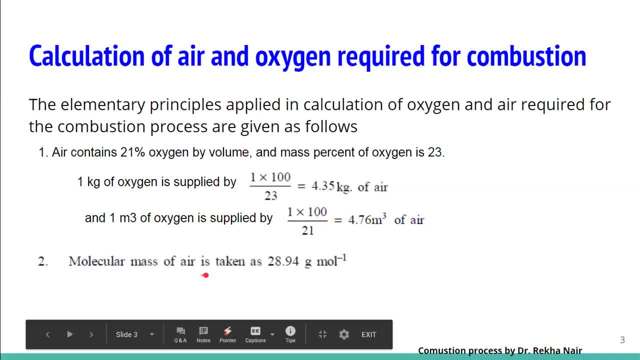 The second assumption that we are making is molecular mass of air is taken as 28.94 gram per mole. The third assumption is minimum oxygen required is equal to theoretical oxygen required, minus oxygen present in the fuel, And the minimum oxygen required should be calculated on the basis of complete combustion. 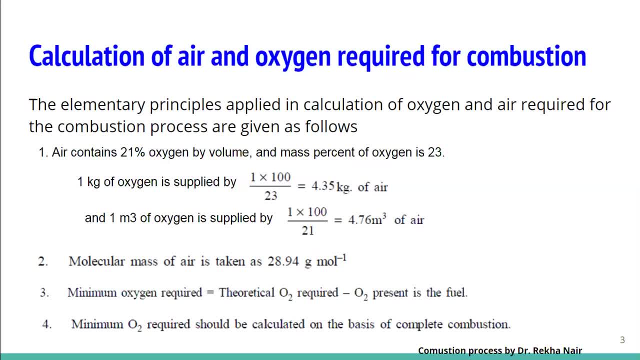 It means that if there is carbon, carbon will react with oxygen to form carbon dioxide. We are not assuming the product as carbon monoxide. The product will be. final product will be always carbon dioxide, because carbon on complete combustion forms carbon dioxide, not carbon monoxide. 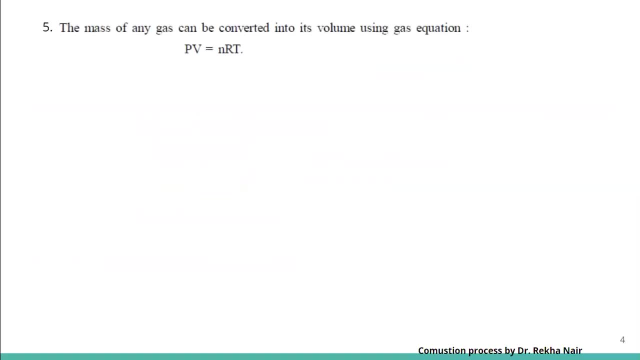 The next assumption is: mass of any gas can be converted into its volume by using the gas equation. PV is equal to NRT, where P is pressure of gas in atmosphere, V is a volume, M is the volume of gas in liters and N is the number of moles of gas and T is the temperature in terms of Kelvin. 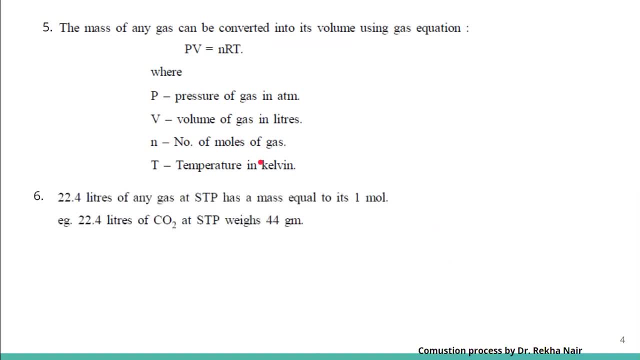 The next elementary rule is: 22.4 liter of any gas at STP has a mass equal to its one mole, That is 22.4 liter of any gas, for example carbon dioxide. its molecular mass is 44. So 22.4 liter of carbon dioxide STP at STP will weigh always 44 grams because its mass is 44.. 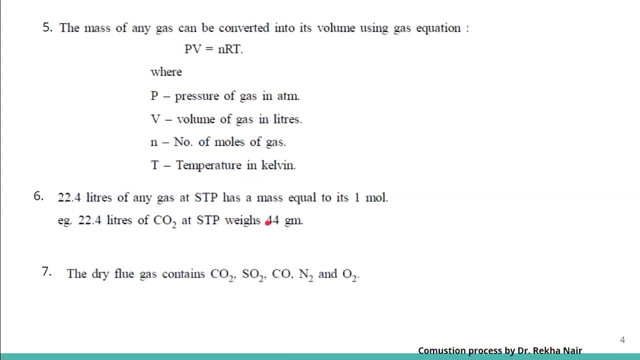 The dry flue gases are carbon dioxide, SO2, CO, N2 and O2.. CO2 and N2 requires no oxygen because it does not undergo. CO2 and N2 need oxygen because it does not undergo. CO2 and N2 require no oxygen because it does not undergo. 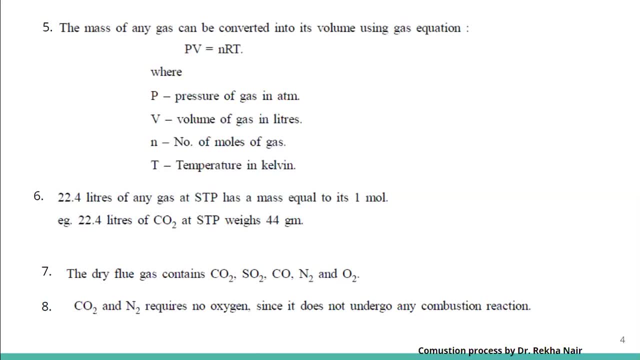 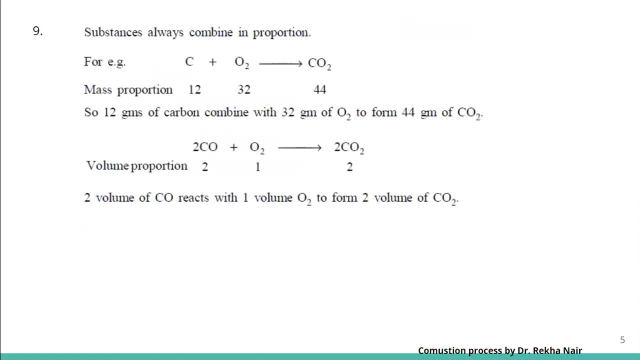 CO2 and N2 require no oxygen because it does not undergo any combustion reaction, that is, it do not have any reaction with oxygen. the next elementary rule is substances always combine in proportion, for example, if we have C plus, or to give rise to CO2 in terms of mass, if we consider 12 gram. 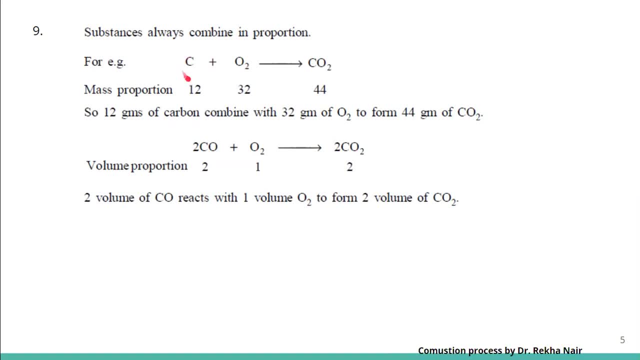 of carbon. carbon atomic mass of carbon is well and that of oxygen. molecular mass of oxygen is 32. molecular mass of carbon dioxide is 44. then we can say that, in terms of mass proportion, 12 grams of carbon will react with 32 grams of oxygen to form 44 gram of carbon dioxide. in terms of volume, we can: 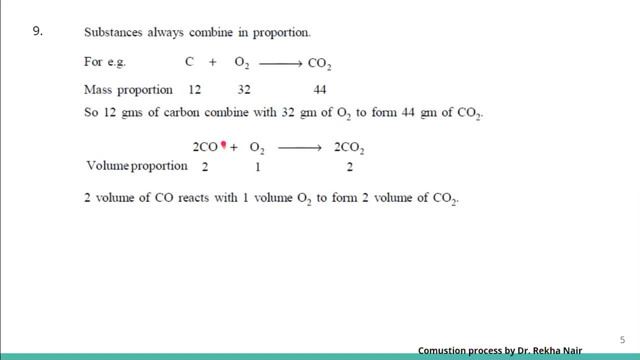 say- we can take another example, for example, 2 CO plus O2 giving rise to 2 CO2. in this case there are 2 COs here and the volume here it is the number of moles, 1, and here the number of moles are 2. so we can say that 2 volume of carbon. 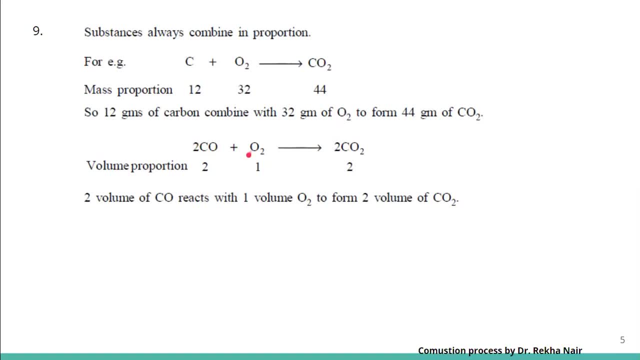 monoxide will react with 1 volume of oxygen to form 2 volume of carbon dioxide. the chemical equations expressing the combustion of some of the constituents. let us discuss, as I already discussed, that carbon will react with oxygen to form carbon dioxide. that is, the complete combustion will take place, and in terms 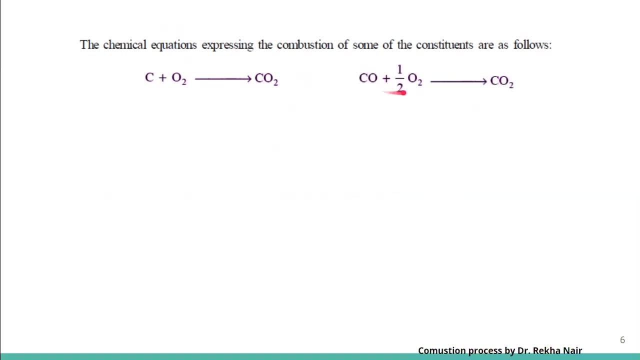 of carbon monoxide. carbon monoxide also will form the product carbon dioxide, so iil utl. its required to come from CO2.. half oxygen to form carbon dioxide. another example is hydrogen. if you have hydrogen, two hydrogen will form one water molecule. so for balancing the 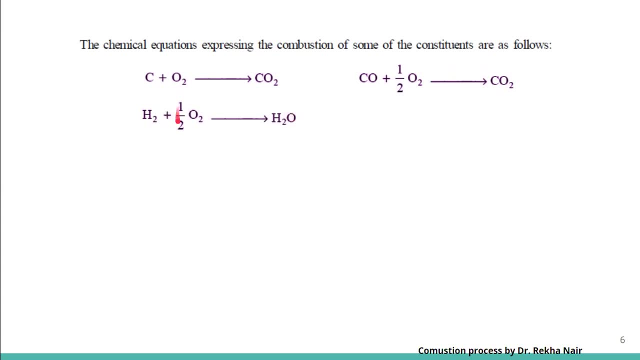 oxygen. here there is one oxygen, so we write it as half oxygen. so hydrogen will react with half oxygen to form water. similarly, if we have methane, there is one carbon will form one carbon dioxide and there are four hydrogens, it will form two water molecules. so in total there are two plus two, four oxygen. so to 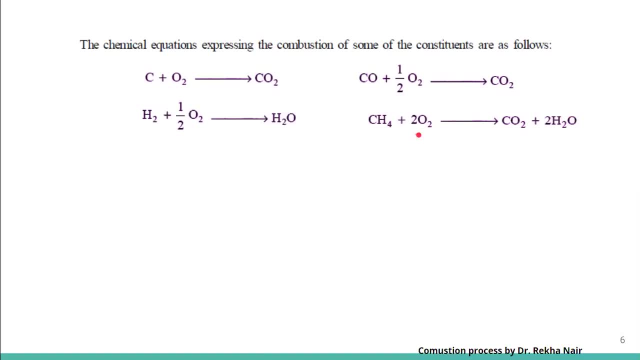 balance, that we write it as CH4 plus two O2. for sulfur it will form sulfur dioxide. so it requires O2, will react with S plus O2. here there are two carbons- it will form carbon dioxide, and that are for hydrogens: it will form two water. 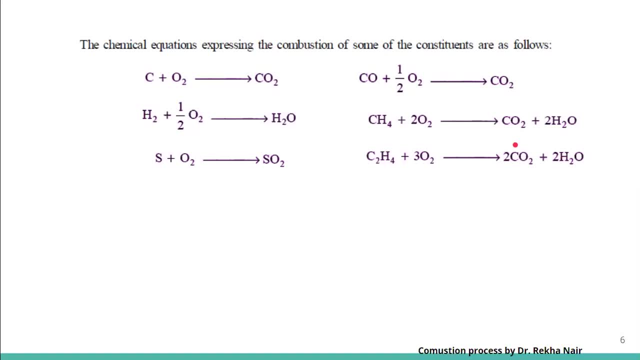 molecules, so four plus two, six oxygens are present here. so via creating it with three oxygen, c2, h4 plus 3, 0, that is 6 oxygen to form the product. in terms of C2H6, there are two blocking atoms will form two carbon dioxide, six hydrogen will form three water. so there 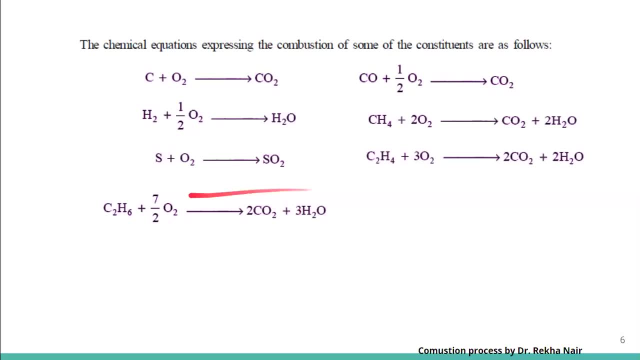 are seven oxygen. in the right hand side we can write it as seven by two or two, plus sequences in terms of C: 3, 8, H, 8. if we discuss, there are three carbon, it will form three carbon dioxide. there are eight hydrogen, so it can form four water. 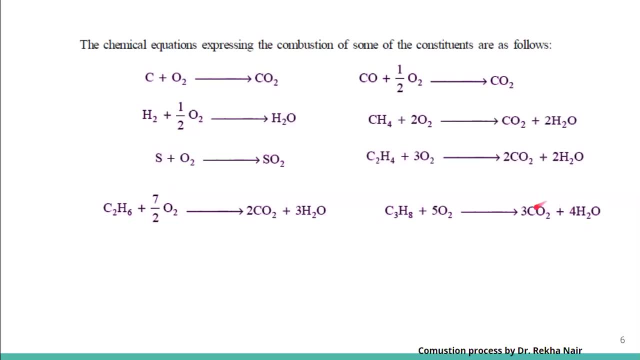 molecules. so in total there are ten oxygens in the right hand side. so there should be. it should be related with five or similar the case with C 2, H 2. there are two carbon formed carbon dioxide, there is two. there are two hydrogens. it 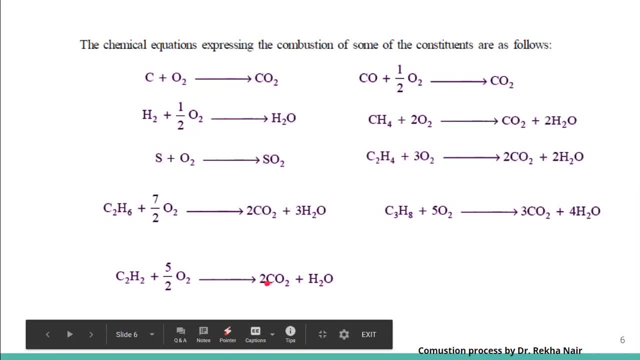 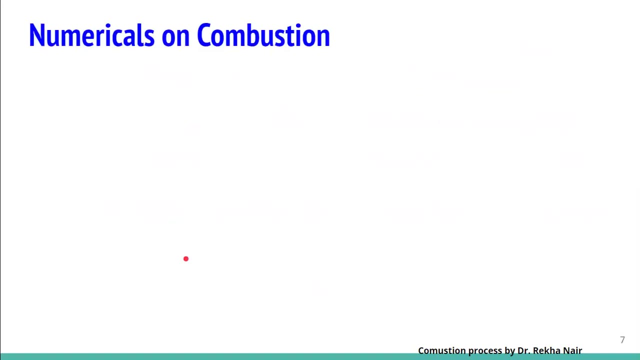 will form one water molecules. so there are four plus one one. five oxygens are there, so here also we need five oxygens, so it is written here as 5 by 2. now let us discuss the numericals on the combustion process. this is the first numerical, the 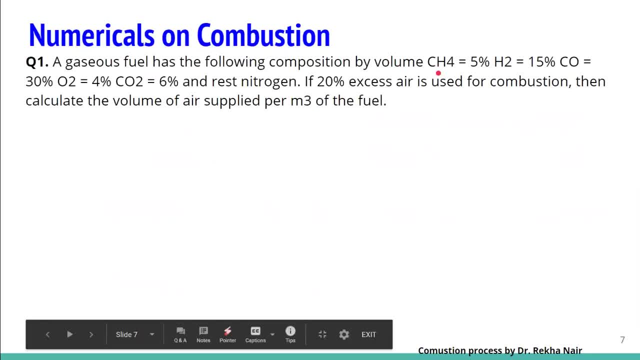 gaseous fuel has following composition by volume: ch4, 5 percent hydrogen, 15 percent carbon monoxide, 30 percent oxygen, 4 percent carbon dioxide, 6 percent and rest is nitrogen. if 20 percent excess air is used for combustion, then calculate volume of air per meter cube of the fuel. 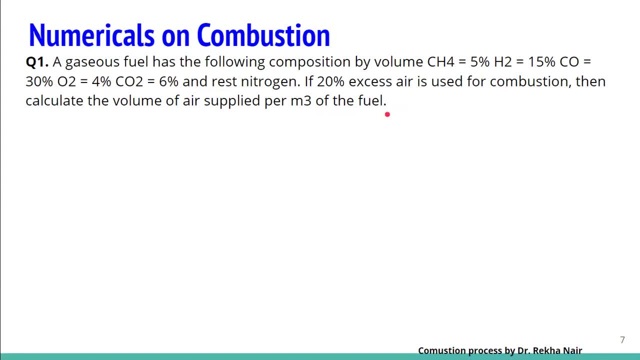 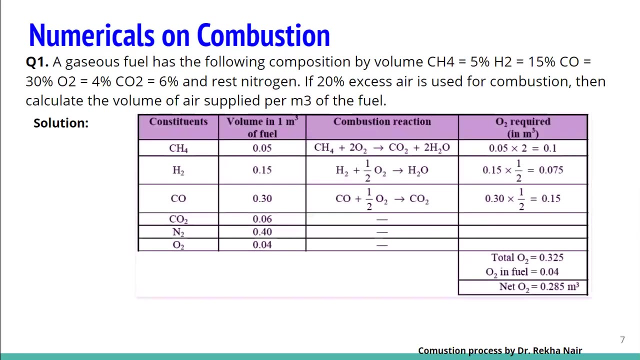 so we are doing the calculation in terms of volume because it is a gaseous fuel and we need to calculate the volume of the air in terms of meter cube. now let us discuss the table. we have all these constituents. given ch4 is 5 percent, so in 1 meter cube of fuel there will be 0.05 meter cube of methane. that is 5 divided. 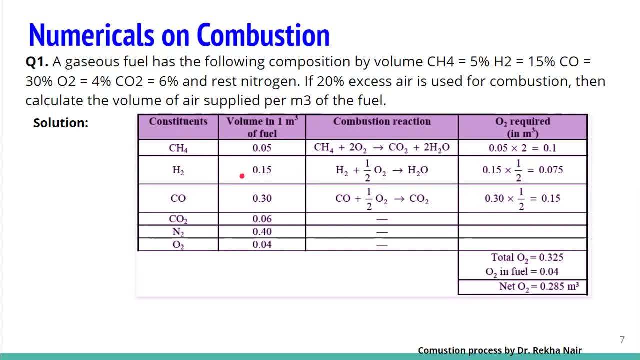 by 100. similarly, hydrogen is 15 percent. so 15 upon 100 is 0.15. so for 100 meter cube it is 15, for 1 meter cube it is 15 upon 100. similarly, carbon monoxide is 30 percent, means for 100 meter cube it. 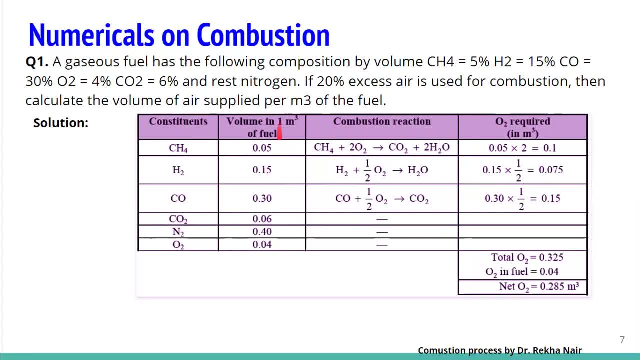 is 30, but for 1 meter cube of fuel it is divided by 100, that is 0.30. similarly, for carbon dioxide is 0.06, nitrogen it is 0.4. oxygen, it is 0.04. so the given percentages are divided by 100 to get the 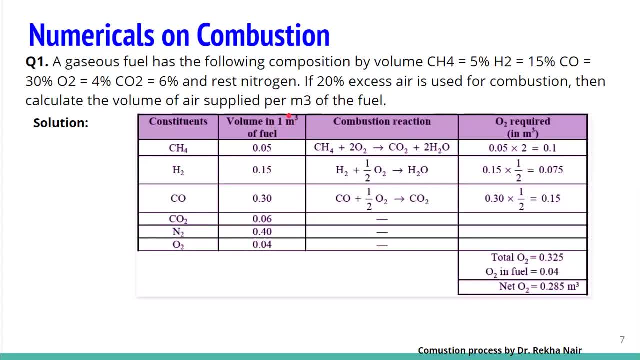 volume in the 1 meter cube of fuel. now let us go for write the combustion reactions. we have ch4. ch4- 1 carbon will form 1 carbon dioxide. there are 4 hydrogen, so it will form 2 water molecules. so number of oxygen present in the right side of the equation are 4, so we need to treat it with 2. 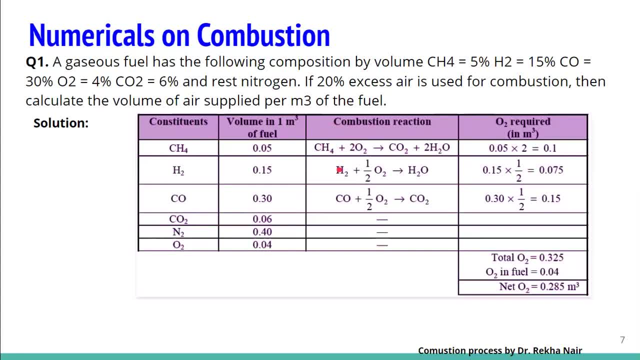 oxygen. in case of hydrogen h2 will form water. so there is 1 oxygen here, so we are treating it with 1 oxygen, that is half o2. carbon monoxide will form the product as carbon dioxide, so we need one more oxygen. so we are writing it as half o2 and we know that carbon dioxide, n2 and o2- all these constituents do not. 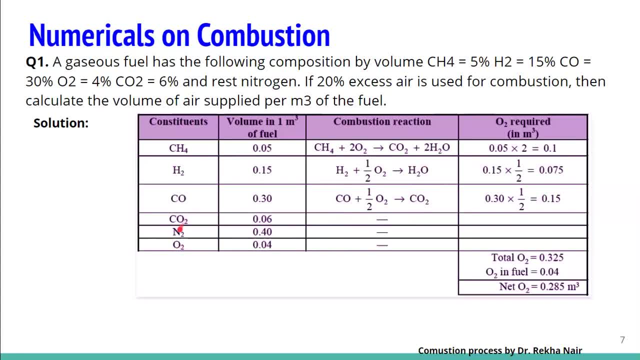 react with oxygen. there is no combustion reaction for these three constituents, so we are not writing them. let us now calculate the amount of oxygen required in meter cube. so the amount of oxygen required is equal to the amount 0.05 that is there in the fuel, multiplied by the number of oxygen as per combustion reaction. so 0.05 into 2 is 0.01. 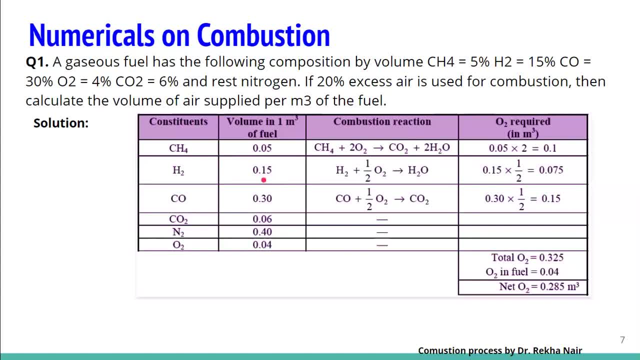 in terms of height in. for hydrogen we have 0.15 meter cube multiplied by half of oxygen, giving 0.05- 0.075. similarly, for carbon monoxide we have 0.30 as quantity and here we are having half of oxygen. so we get 0.15 as required oxygen. for carbon dioxide, nitrogen and oxygen there is. 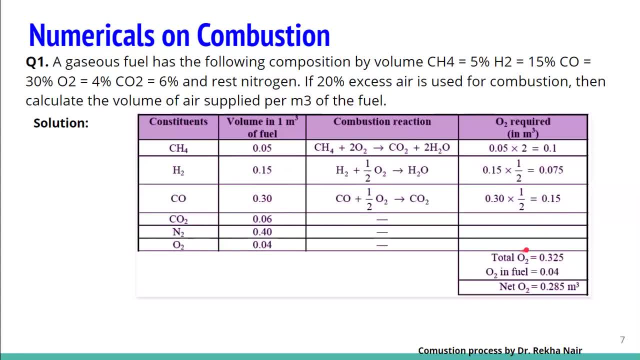 no reaction with oxygen, so it will not consume any amount of oxygen in the combustion process. so we can total all these three quantities. we get 0.325 meter cube now, but oxygen is already present in the fuel. this amount of oxygen present in the fuel must be subtracted to get the actual oxygen required for the combustion process, so net. 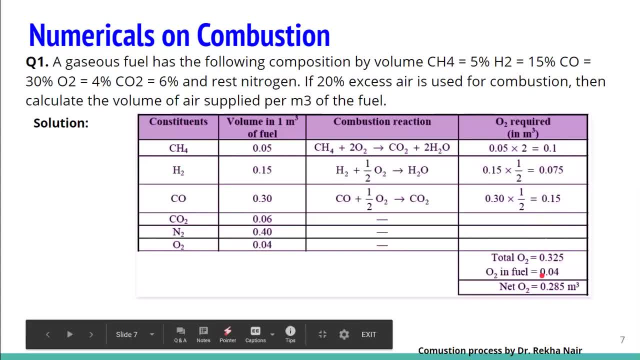 oxygen is equal to 0.325 minus 0.04, equal to 0.285 meter cube. if you want to calculate the minimum volume of air required, then oxygen multiplied by 100 upon 21 will give the amount of air required. so 0.285 multiplied by 100 upon 21 will give 1.35 meter cube of air. so the minimum 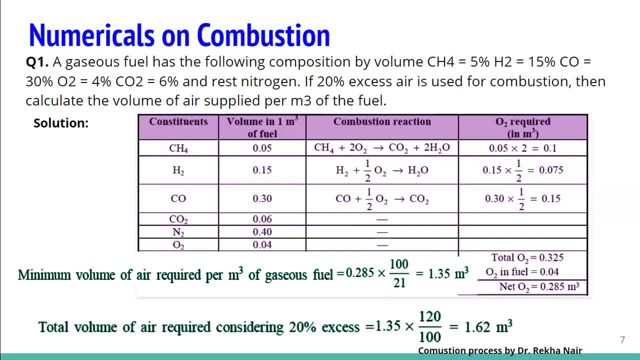 volume of air required is equal to 1.35 meter cube. so but in question it is given that there is 20, 20 percent of excess air used for the combustion. so total volume is equal to. we have to calculate for 120 percent, that is, 1.35 multiplied by 120 percent will give 1.62 meter cube. so this: 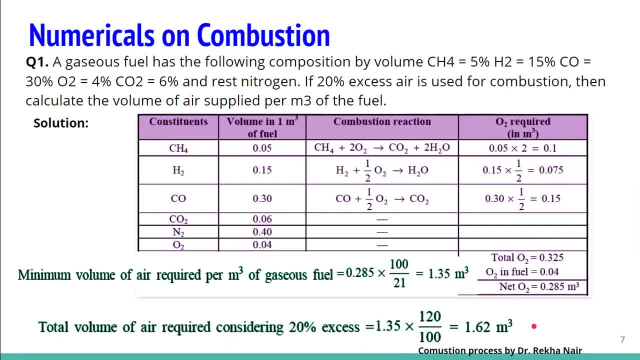 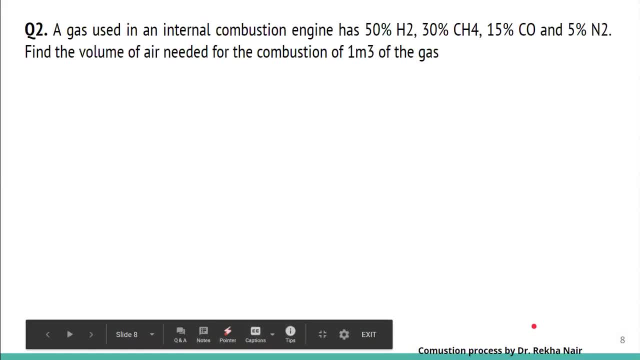 is a total volume of the air required by considering 20 percent excess air. let us discuss another numerical. a gas used in an internal combustion engine has 50 percent hydrogen, 30 percent methane, 15 percent carbon monoxide, 5 percent nitrogen. so again it is a cache screen and asking for find the volume of air needed for combustion of. 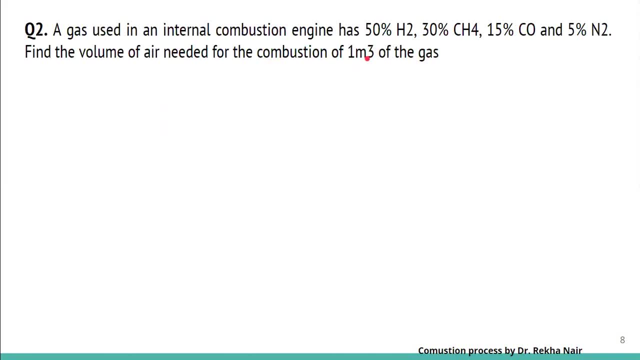 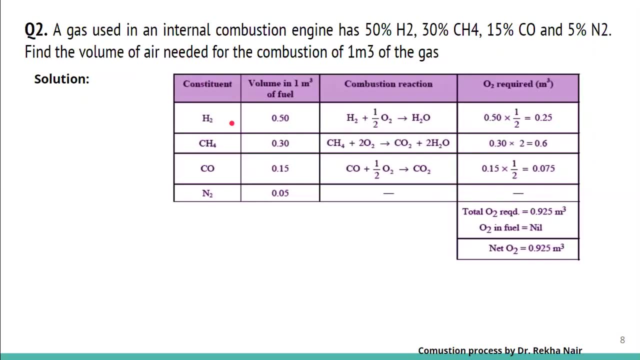 one meter cube of the gas. so again we are doing the calculation in terms of volume. let us discuss another numerical: a gas used in an internal combustion engine has 50 percent hydrogen, 30 percent, than the gas used in another mechanical plant. again we have to make anаго table having constituents as given and 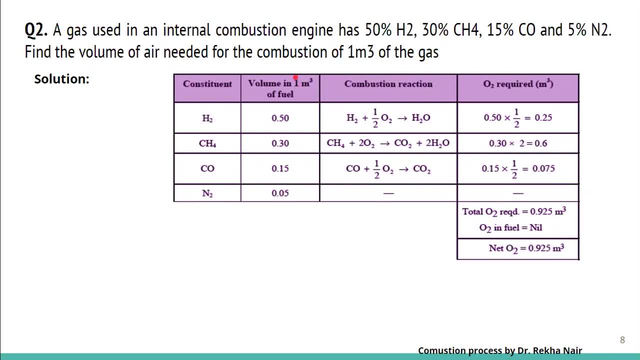 this is a volume in terms of 1 meter cube because they are asking for point, the volume of air needed for 1 meter cube and we are having the percentages of the constituents. we have to divide these percentages by 100 to get volume in terms of 1 meter cube. so in 1 meter cube hydrogen is 50 divided by hundred. 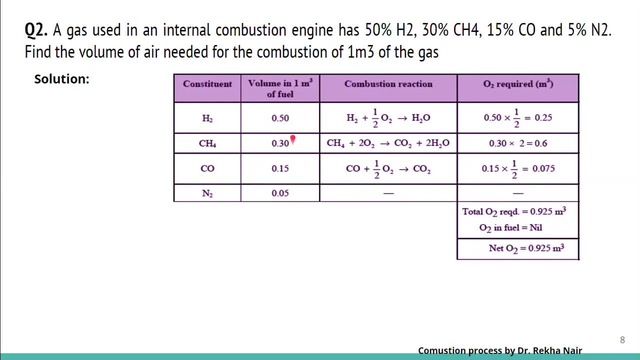 50. 30 divided by 100.30 is methane. for carbon monoxide 15 divided by 100.15. and nitrogen is given as 5 percent. so 5 divided by 100 is 0.05. now let us discuss combustion reaction of this. 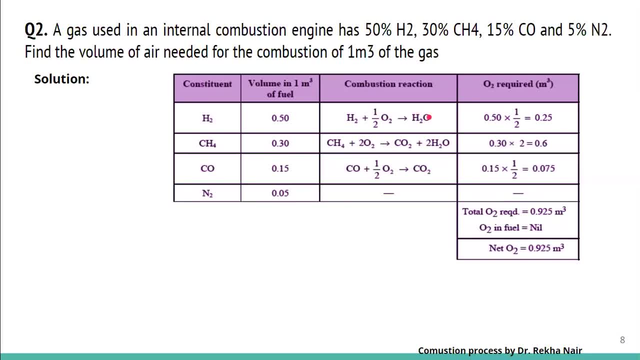 hydrogen will give water, so it needs one oxygen. so half o2 methane, one carbon, will form one carbon oxide. four hydrogen will form two water molecules. so there are four oxygens in the right hand side of the equation. so to balance that we are writing it as 2 o2, that is for oxygen similarly carbon. 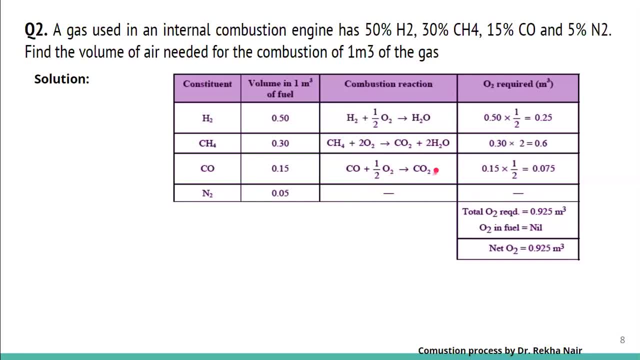 monoxide will react with half of oxygen to form carbon dioxide. as i have already discussed, the amount of oxygen required will be calculated by the volume in one meter cube of the fuel multiplied by the number of oxygen required for the combustion. so 0.50 multiplied by half will be 0.25 meter cube and in this case 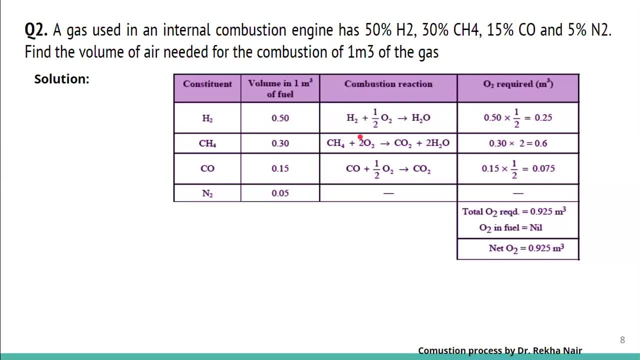 0.30 multiplied by 2 will give 0.06 meter cube and 0.15 multiplied by half will give 0.075 meter cube. total oxygen required is 0.925 meter cube. there is no oxygen given in the fuel, so we don't need to. 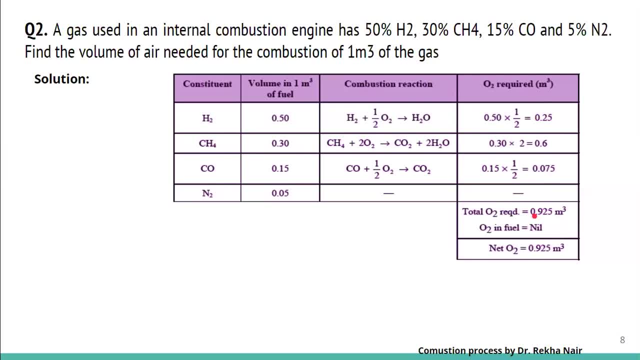 do that. so oxygen fuel is nil, so net oxygen will be equal to 0.925 minus 0, that is 0.925. the volume of the air required for one meter cube of gas will be 0.925 multiplied by 100 upon 21, because there 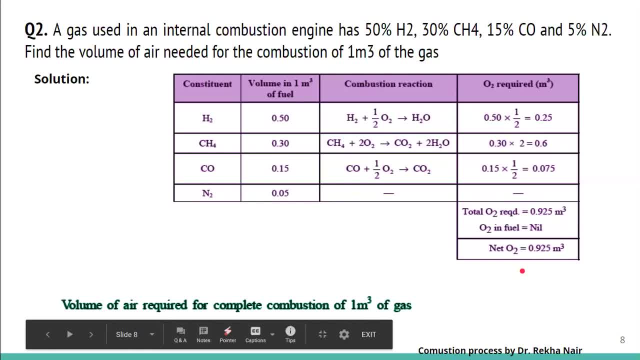 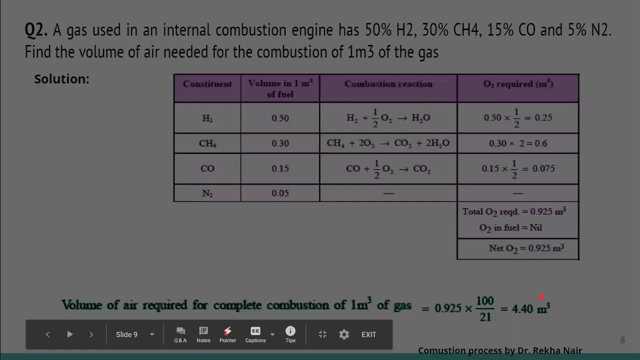 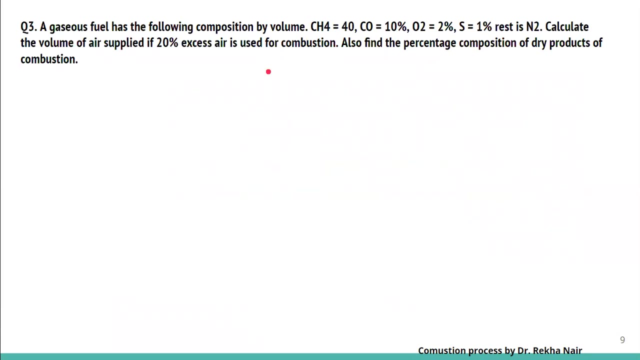 is 21 percent of oxygen by volume in the air, as i have discussed in the elementary principle number 1, so it will come out to be 0.925 into 100 upon 21 equals to 4.40 meter cube. now let us find out. let us discuss another numerical here. it is given that a gaseous 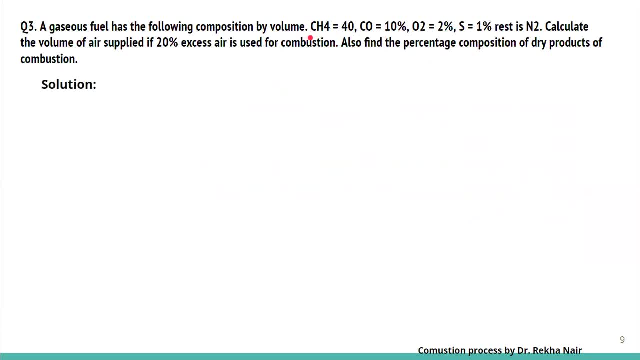 fuel has following composition by volume. so it is a gaseous fuel and we are calculating in terms of volume again: ch4 40 percent, carbon monoxide 10 percent, oxygen 2 percent, sulfur 1 percent and rust is nitrogen. calculate the volume of air supplied if 20 percent excess air is used for. 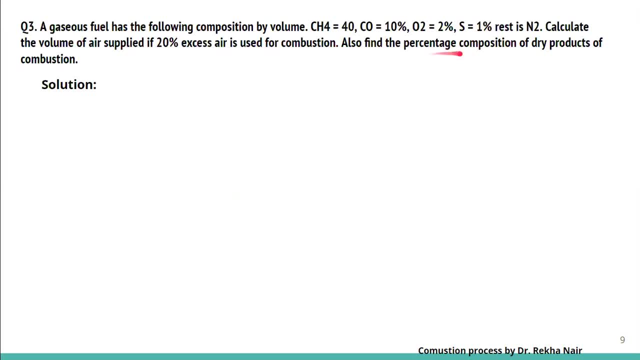 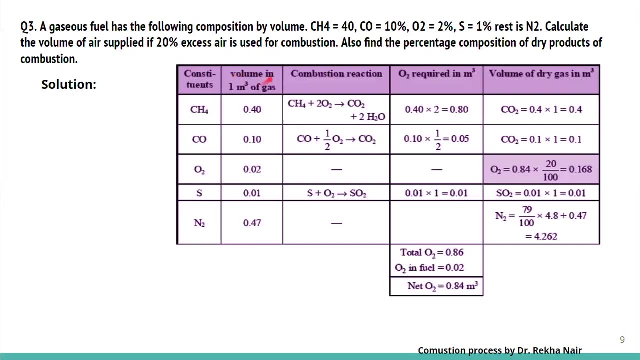 combustion, also find percentage composition of dry products of the combustion. now let us discuss the table here also. we are calculating for one meter cube of the gas, because it has been asked that we need to calculate the percentage composition. we are calculating for one meter cube, So for 1 m3, 40 divided by 100, carbon monoxide is 10 divided by 100, oxygen is 2 divided by 100,. 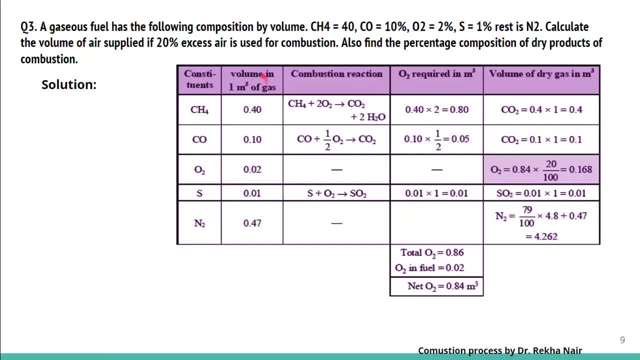 sulfur and nitrogen. all this we are calculating in terms of 1 m3 of gas. Now let us discuss about combustion reaction. We have CH4, 1 carbon gives 1 carbon dioxide and 2 water molecules, because 4 hydrogen will react to form 2 water molecules. 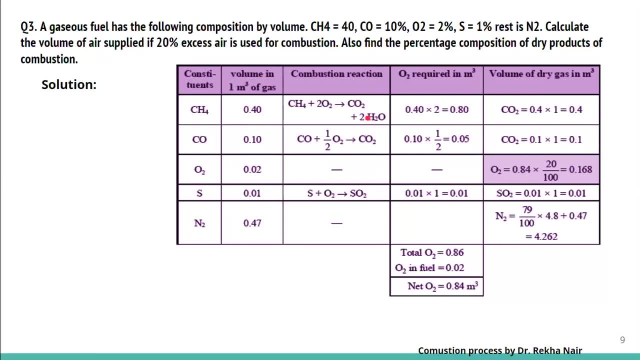 So total number of oxygen required is 4 in the right side. so we are treating it with 2 O2.. Carbon monoxide will form carbon dioxide. it requires 1 more oxygen, so half O2.. Oxygen has no combustion reaction. sulfur will react with oxygen to form SO2,. 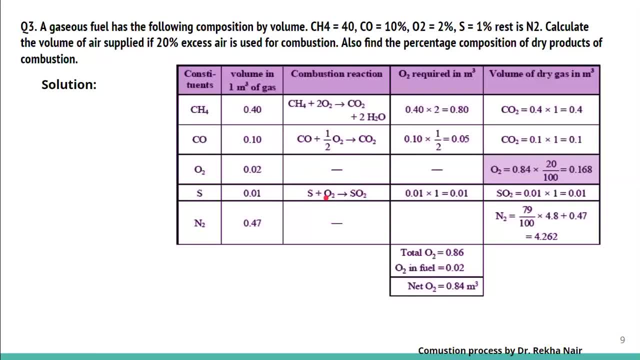 it requires 2 oxygen, so it is treated with 2 oxygens. Nitrogen does not undergo any combustion reaction, so we do not have any combustion reaction. for this, Oxygen required will be equal to 0.40. multiplied by number of oxygen is 2 equal to 0.80.. 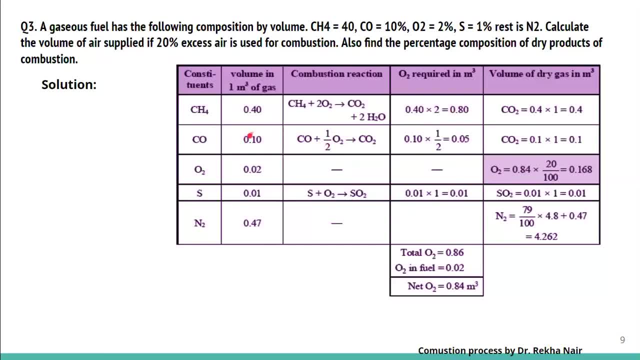 0.10 is a volume multiplied by half is equal to 0.05.. Oxygen is not required for O2 and for sulfur it is 0.01,. multiplied by half is equal to 0.05.. Oxygen is multiplied by 1, oxygen gives 0.01.. 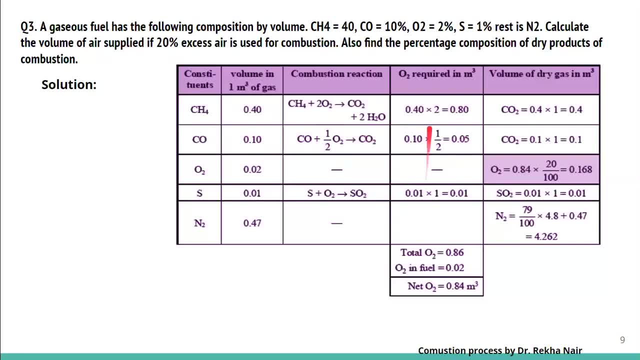 In case of nitrogen, it requires no oxygen. so we are calculating total oxygen as 0.86.. 0.80 plus 0.05 plus 0.01, that is 0.86.. But oxygen is there in the fuel as 0.02 m3 in 1 m3.. 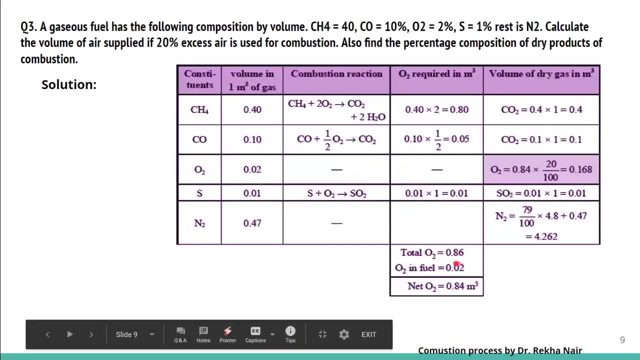 So we are subtracting 0.02 from the total oxygen, we get net oxygen 0.02 from the total oxygen, we get net oxygen 0.02 from the total oxygen, we get net oxygen 0.04 m3, and volume of air is equal to 0.84 multiplied by 100 upon 21, that is 4 m3. 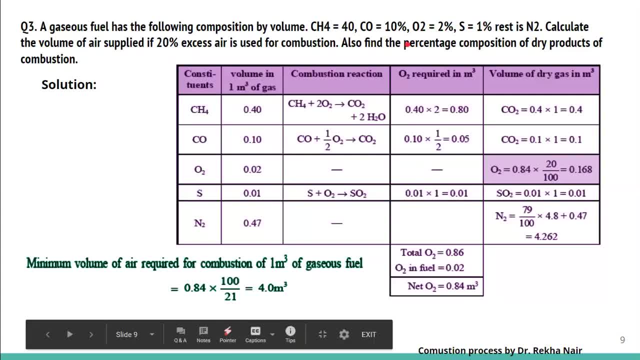 Now they have also asked to find out the percentage composition of the dry products of combustion. See, here, dry products means we have to consider only carbon dioxide. Water is not required, not a dry product. so we are calculating the volume of carbon dioxide in this case. to calculate volume. 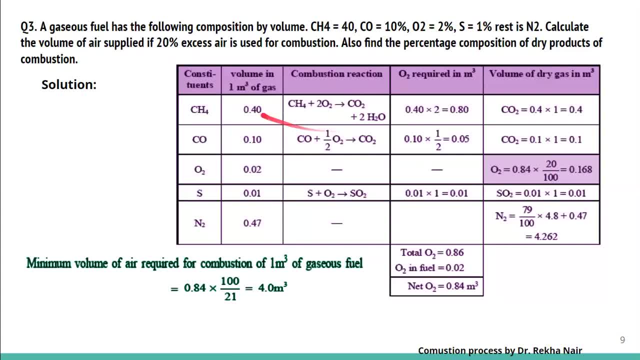 of dry gas carbon dioxide, we multiply 0.40 multiplied by number of carbon dioxide, that is one. so we get 0.4 multiplied by 1, equal to 0.4. in the second case we have one carbon dioxide again, so 0.10 multiplied by the product that is dry product, that is, from this carbon dioxide one. 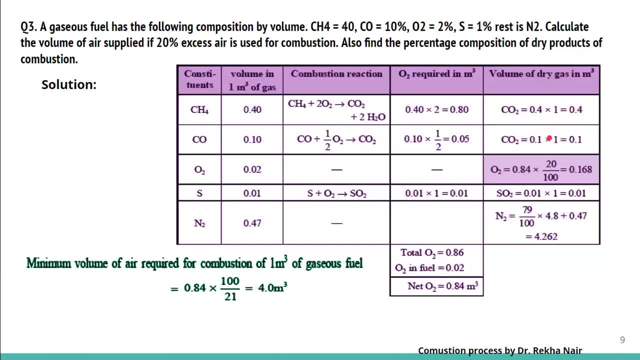 molecule, so we multiply it by one. in case of oxygen, what we need to do is we have to multiply 20 percent because we have- they have given it- as 20 percent excess air is used for the combustion. this 20 percent here has whatever amount of oxygen that will be going. 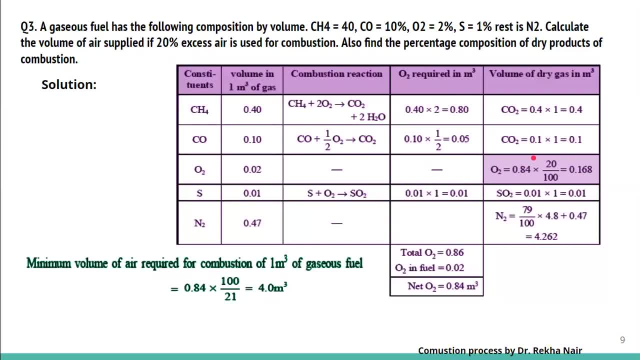 through gases or dry gases that will be removed in the through the chimney. so what we need to do is the net oxygen is 0.84, for the 20 percent of 0.84 is equivalent amount that will be lost in the process as dry gas that this, this oxygen, also will be. 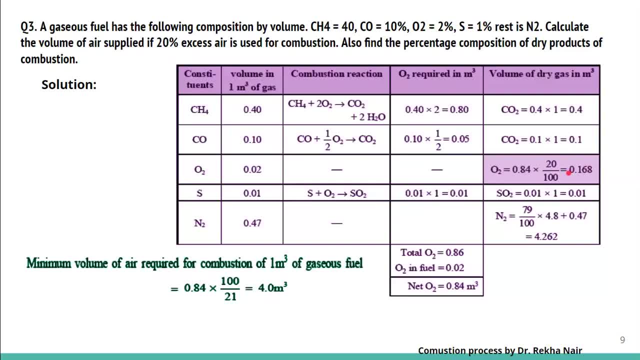 removed through chimney like carbon dioxide. only 100 percent of the oxygen will be calculated in the oxygen natural gas. so this is the total of the carbon dioxide that we have again. so now we have to face is the fluid which is produced here. so we need to overcome the 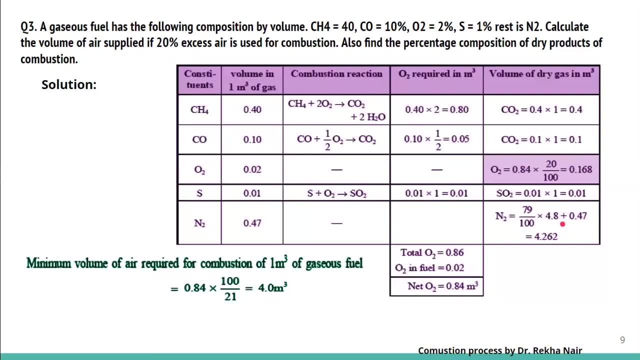 nitrogen suggested oxygen as well as nitrogen. managers x. the products that we have similar in is nitrogen. okay, 79 percent of air is nitrogen, so 79 percent of total air. we have calculated as 4.0, so you have to write it as 4.0. it's not 4.8, it's 4.0. 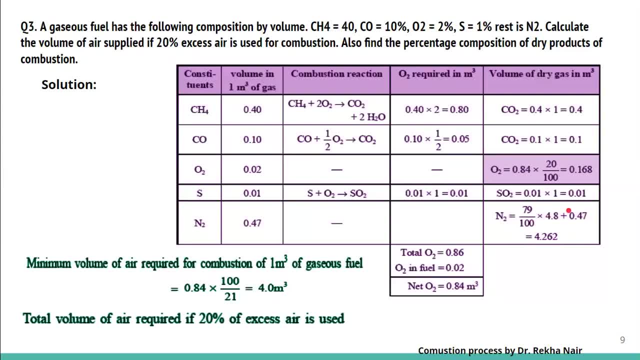 plus 0.47 is already present in the fuel. so this amount present in the fuel that is not reacting with anything, that will also mean that also will go as a flue gas and 79 percent of the air contains nitrogen, so that also will go in the. 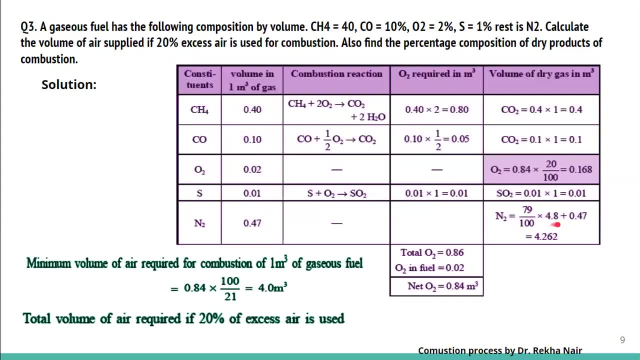 flue gas. so the total amount of nitrogen that will be removed as dry product as four point two six two seventy nine percent of 4.0 plus 0.47 will give four point two six two meter cube. if there is excess of air, twenty percent of excess. 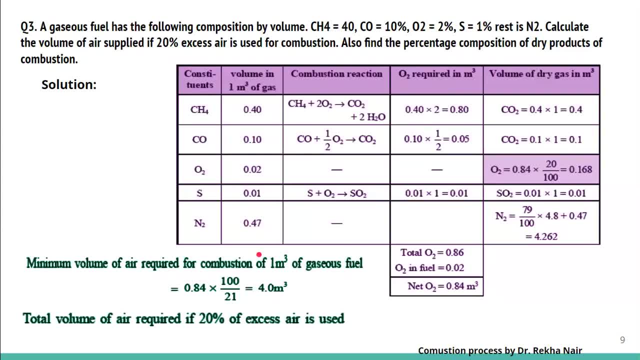 of air is given, so we have to calculate for it twenty percent of excess of air. so twenty percent of excess of air will give one twenty percent as four point eight. in that case what we have to do is the total nitrogen that is going waste is not four point zero, it should be. 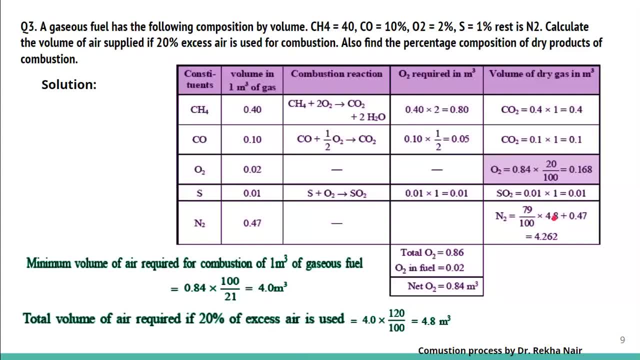 calculated as four point eight. so it is written as four point eight here because in the question it is given that there is twenty percent of the excess air that is being used for the combustion, the whole amount of nitrogen will go waste. if there is no percentage excess is given, we need to calculate only total. 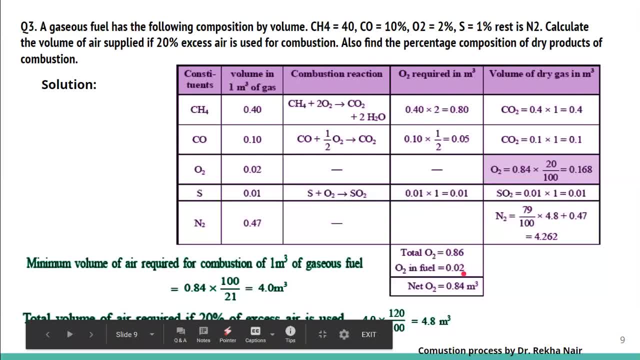 amount of air, that is four point zero. in this case there is excess air is given, so the total volume of air is coming out to be four point eight. so nitrogen will be seventy nine percent of four point eight plus point four seven. that is already in the fuel, the whole nitrogen. 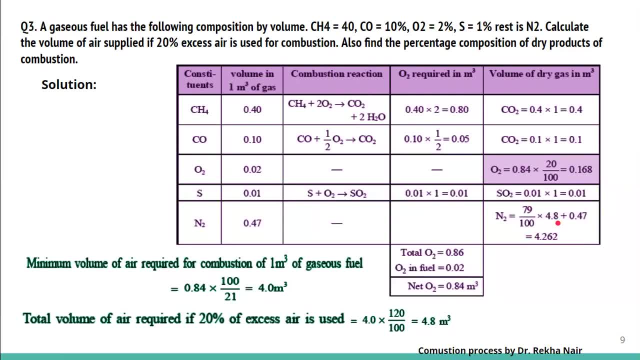 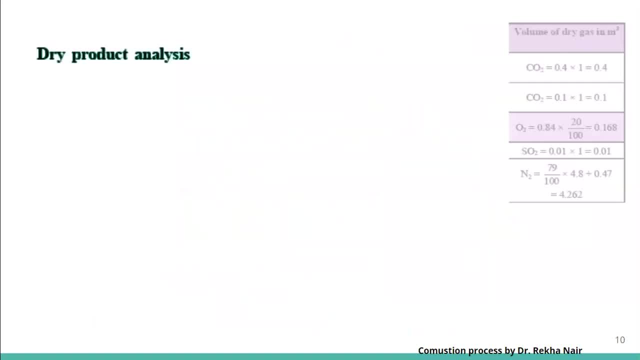 will go as flue gas. now let us calculate the percentage of the oxygen that is going to be. this is given to us in the dry products form. this is a. this is a as per table given. so total volume of carbon dioxide is equal to point four plus point one, that is, point five. 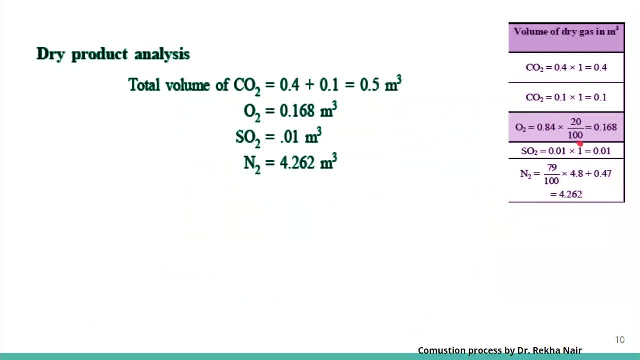 meter cube. oxygen we have calculated as point eight. four multiplied by whatever excess percentage is given, that is twenty percent, and SO2 as point zero one and nitrogen is coming out. So we need to calculate the percentage of all the amount. percentage is equal to total. 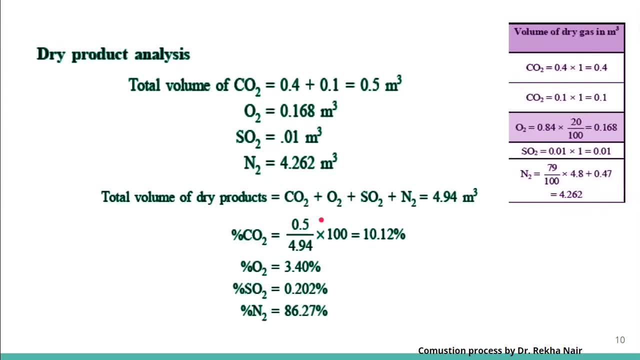 volume is 4.94,. so percentage carbon dioxide is equal to amount of carbon dioxide 0.5 multiplied by total volume of the dry products multiplied by 100.. So 0.5 divided by 4.94, multiplied by 100, is a percentage. 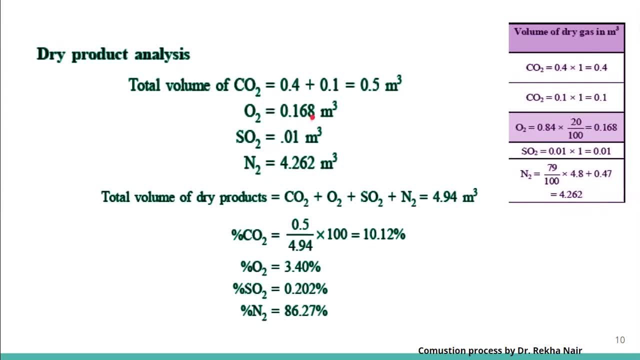 Similarly, oxygen is 0.168 divided by 4.94 is a total volume multiplied by 100.. Similarly, SO2 is 0.01 divided by 4.94, multiplied by 100.. Nitrogen is 4.262 divided by 4.94. multiplied by 100 is 86.27.. 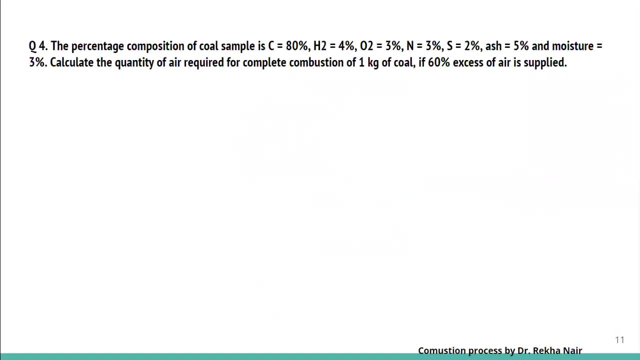 Now The next, let us discuss next, numerical. the percentage composition of cold sample is. so we are having a solid fuel, cold sample. It's not a gaseous fuel. The first observation is that it is a solid fuel, So we have to calculate in terms of mass instead of volume. Carbon is 80%, Hydrogen 4%, Oxygen 3%, Nitrogen 3%, Sulfur 2%, Ash 5% and Moisture 3%. Calculate the quantity of air required for complete combustion of 1 kg of coal. 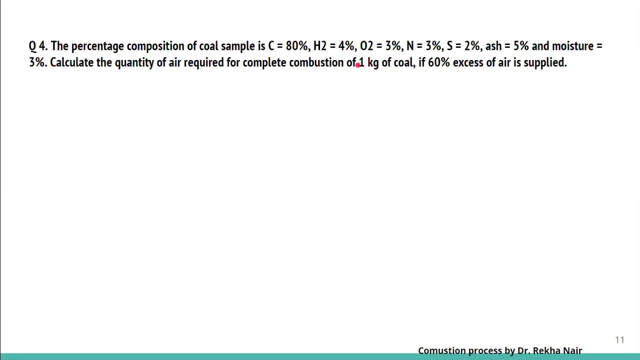 It is not 1 meter cube now, It is the in terms of mass, So 1 kg of coal, and if 60% excess air is supplied, So we have excess of air also. Now let us discuss the table Here. we are having carbon. 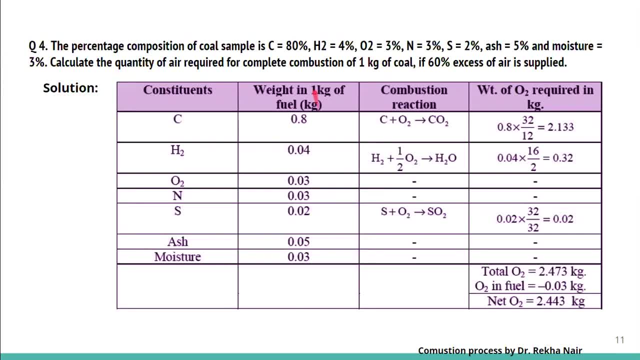 Again, we are calculating for 1 kg of fuel, So this percentages will be converted By dividing it by 100.. So we have 0.8, Hydrogen 0.04, Oxygen 0.03, Nitrogen 0.03.. 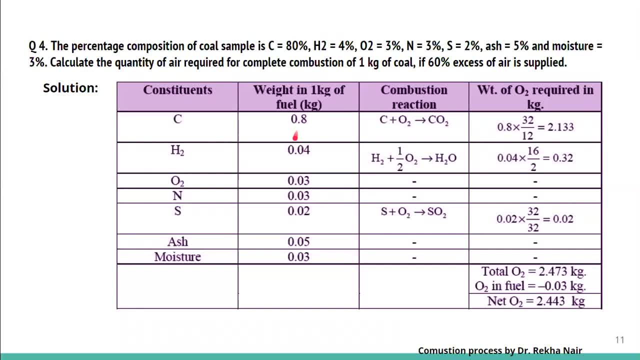 Everything will be. all the percentages will be divided by 100 to get this amount in 1 kg. Combustion reaction is similar as discussed in the volumetric analysis. Carbon will react with oxygen from CO2.. H2 plus half O2, giving rise to carbon. 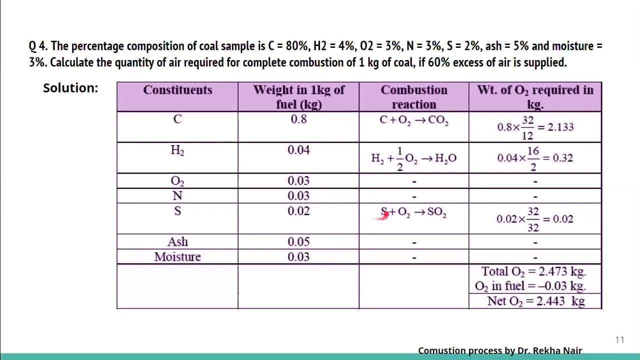 Carbon will react with oxygen from CO2.. H2 plus half O2 giving rise to carbon Carbon will react with oxygen from CO2.. H2 plus half O2 giving rise to carbon Sulfur will react with oxygen to form SO2.. Sulfur will react with oxygen to form SO2.. Now the calculation of oxygen in terms of weight, that is, weight of oxygen, will be calculated in a different way. Here what we have to consider is in terms of proportion, In terms of volume. it was one volume reacting. 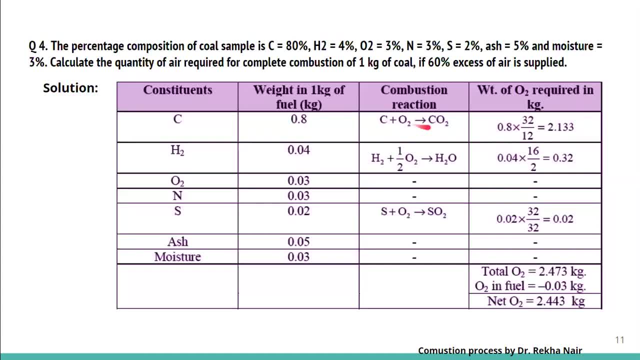 one volume of carbon, reacting the one volume of oxygen to give one volume of carbon dioxide. In terms of mass, what you have to consider is 12 g of carbon will react with 32 g of oxygen to form 44 g of carbon dioxide. 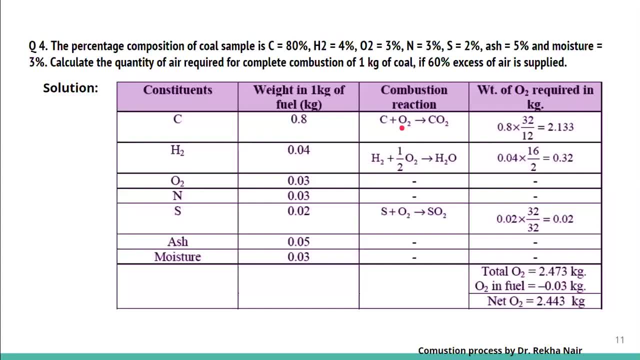 So oxygen required is equal to. we can say that 12 g of carbon requires 32 g of oxygen, So the amount of oxygen required is equal to 0.8 multiplied by 32, divided by 12.. 32 is mass of oxygen. divided by 12 is mass of carbon. 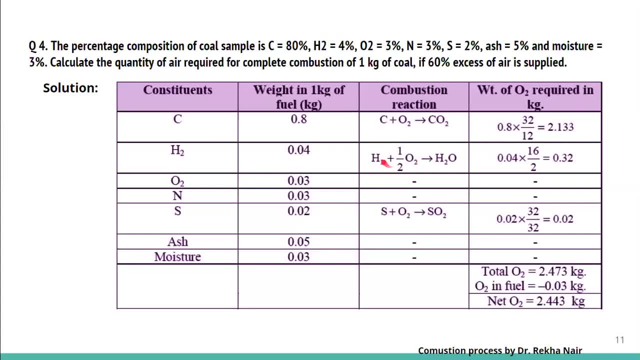 Similarly in this case. if we calculate, we have 2 g of hydrogen reacting with 16 g of oxygen to form 18 g of water. So oxygen required is how much? For 2 g of hydrogen it requires 16 g of oxygen. 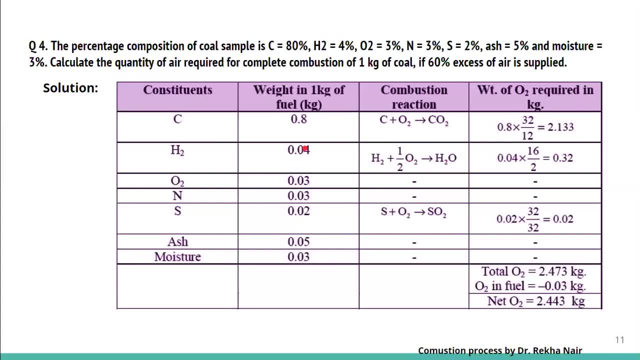 So for 0.04 g of fuel hydrogen it requires multiplied by 16, by 2.. Oxygen do not have any combustion reaction. Nitrogen also do not have any combustion reaction. as I have already discussed, Sulfur is reacting with oxygen to form SO2.. 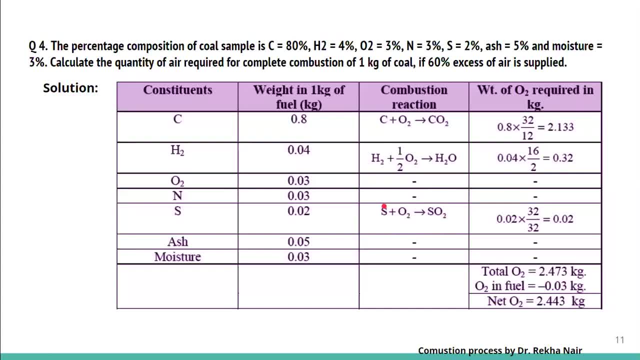 So sulfur is 32. g of sulfur will react with Oxygen is also 32 will form the corresponding SO2.. So 32 g of sulfur requires 32 g of oxygen. So we are multiplying 32 by 32, multiplied by the amount in 1 kg. 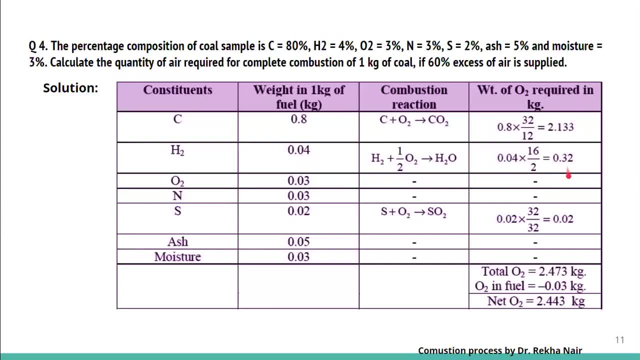 So we are having the oxygen required. So we are totaling all these three quantities to get total oxygen: 2.473.. But oxygen in the fuel As 0.03, we have to subtract this. So we are subtracting it minus 0.03 is equal to 2.443 kgs net oxygen. 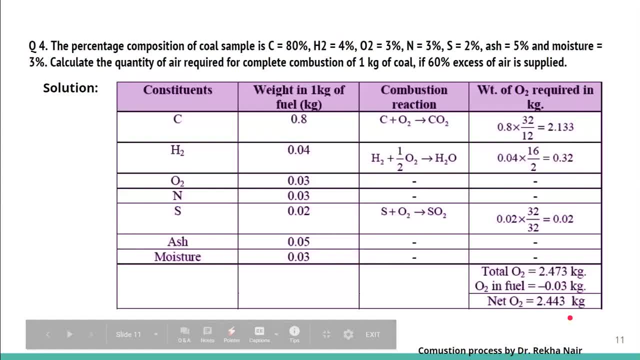 Now we have to calculate the amount of air required, because they are asking for quantity of air required for complete combustion of 1 kg of coal. So the minimum weight of oxygen required is equal to. minimum weight of air required is equal to. This is oxygen required is 2.443. 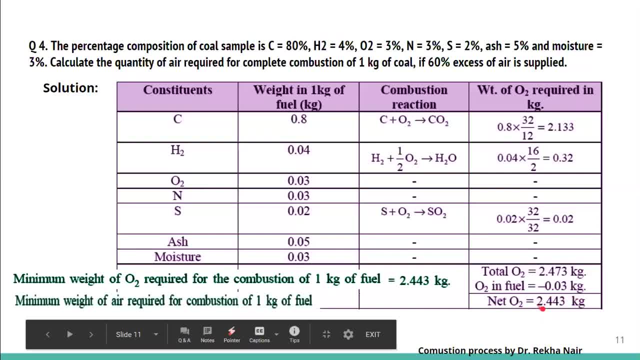 And air required will be equal to 2.443 multiplied by 100 upon 23.. Because, as per principle number 1, I have discussed that there is 23% of oxygen in terms of mass in the air. There is 23% of oxygen in the terms of weight. 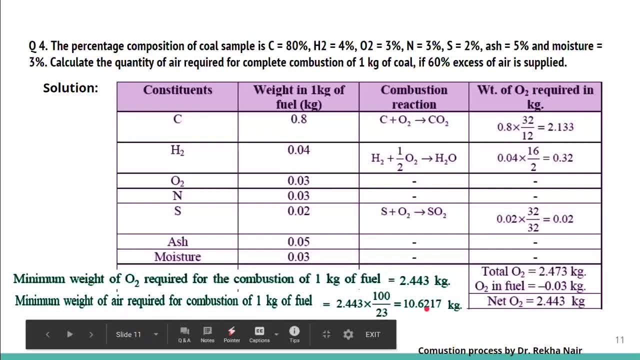 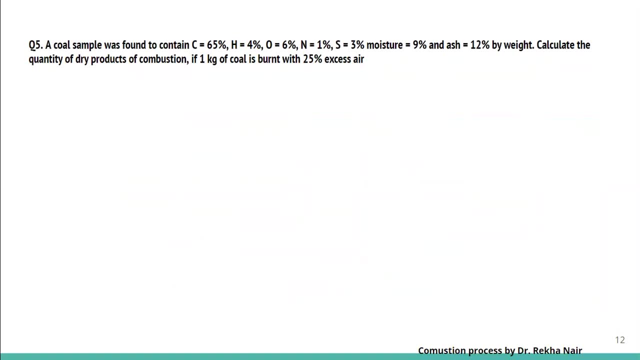 So 2.443 into 100 upon 23.. We get 10.6217 kg. There is 60% excess air supply. So for 160% we have to multiply it with 160%. Next question, number five: Again, a coal sample was found to contain carbon, 65% hydrogen, 4% oxygen, 6% nitrogen, 1% sulfur, 3% more carbon. 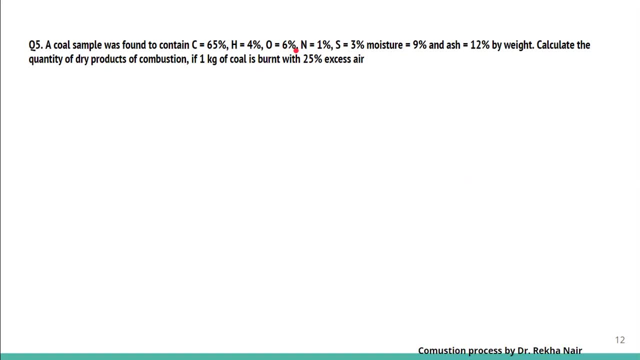 So we have to multiply it with 160%. Next question, number five: Again, a coal sample was found to contain carbon 65%, hydrogen, 4% oxygen, 6% nitrogen, 1%, sulfur, 3% more carbon, So we have to multiply it with 160%. 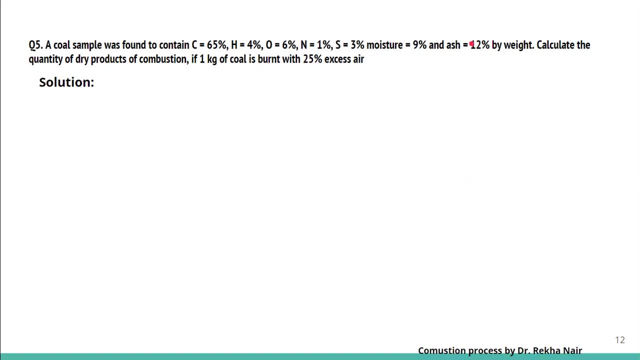 So there is a gas, Moisture, 9%, and ash 12% by weight. Calculate the quantity of dry products of combustion if one kg of coal is burned with 24% of excess air, Here again we are having in terms of mass. 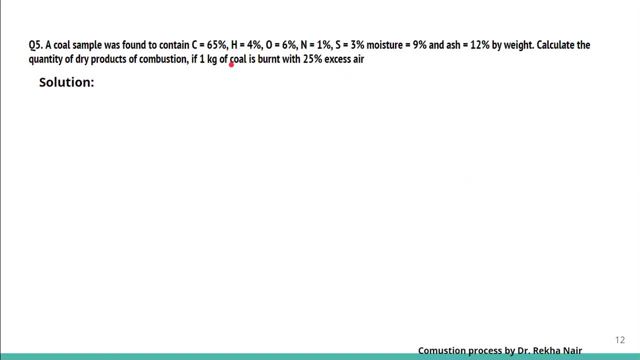 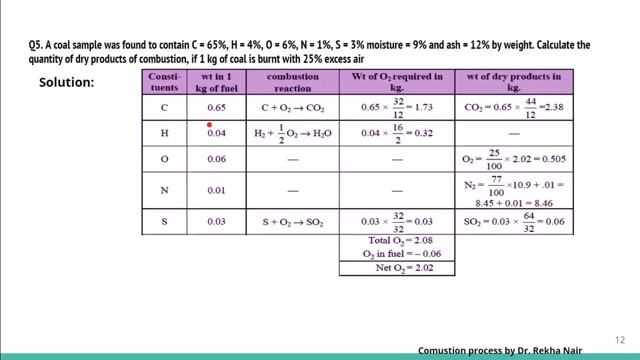 And we have a solid fuel as coal. We have to do the calculation in terms of mass. We have carbon 65%. We have carbon 65% kg divided by 100: 0.65. for hydrogen, it is 0.04 oxygen, 0.06 nitrogen, 0.01 sulfur, 0.03 moisture. 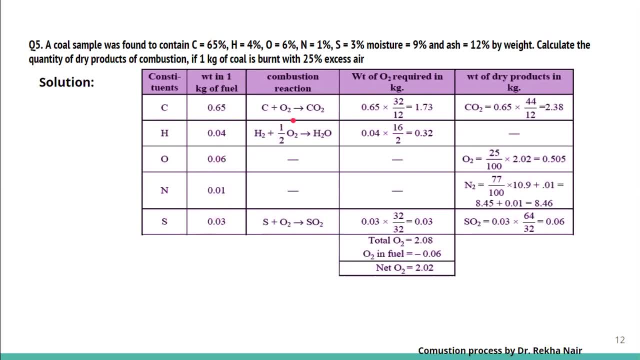 we don't consider ash content, we don't consider carbon will react with oxygen to form carbon dioxide. hydrogen will react with oxygen to form water. for oxygen. there is no combustion reaction. for nitrogen. there is no combustion reaction for sulfur. we have sulfur plus also giving rise to 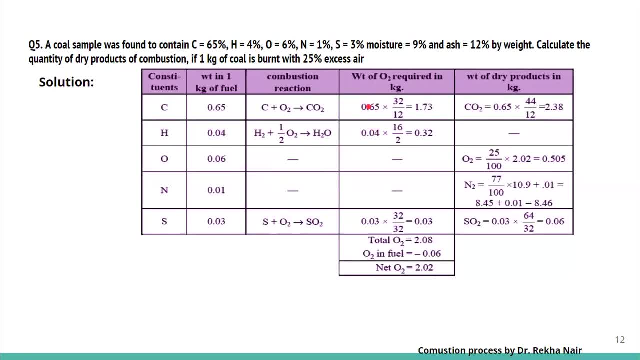 sot. so weight of oxygen required is equal to, again, in terms of mass. i said already, 12 gram carbon requires 32 gram of oxygen. for 0.65 we need multiplied by 32 by 12.. similarly for hydrogen we have two gram. hydrogen will react with half of oxygen, that is 16 gram. so we are multiplying it with 16 by 2.. 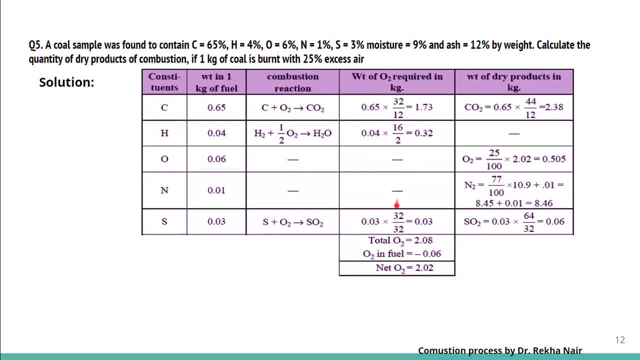 oxygen requires no oxygen in the combustion. nitrogen also has no combustion reaction. sulfur- again 32 gram of oxygen and 32 gram of sulfur. so we are multiplying it with 32 by 32, we are having total oxygen. as we can sum up all these values we get. 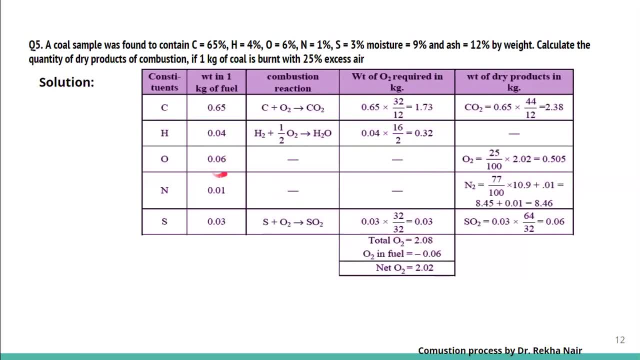 2.08. so oxygen in the fuel is also given as 0.06. we need to subtract it as we did in the volumetric analysis. so net oxygen we have 2.02 kg. now we need to do the calculation for dry products. so, as i said here, the dry product is carbon dioxide. 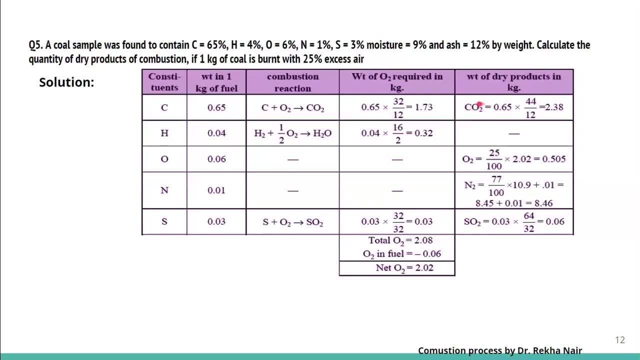 so we need to do the calculation for carbon dioxide. the amount is 0.65 and this carbon- 12 gram of carbon- produces 44 gram of carbon dioxide. so we are multiplying 0.65, multiplied by 44 by 12.. hydrogen forms water, which is not a dry product, so we don't need to. 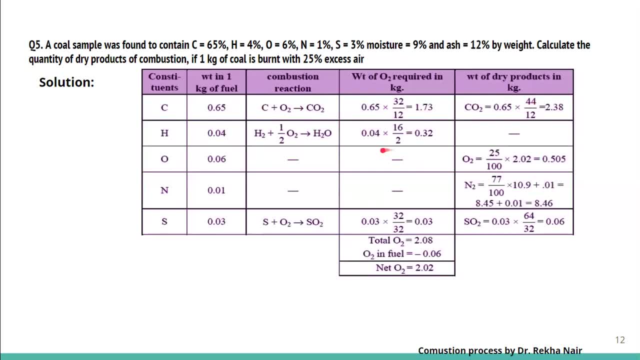 calculate it. oxygen do not undergo any combustion reaction, but since there is 25 percent of excess air is given the amount present in that 25 per как, This distance, 20% of excess air is given the amount present in that 25% of인 that body as given, and we are Ek Cartesian composite of 10% of this Hydrogen of Food CO2 on 30 percent of carbon dioxide. בסl chớ supply 30% X 24- 0.63 percent EVA matters. and after the time this over current temperature increases Sları uda as G stats for the air concentration increases. so we achieve a normal natural Ranian- stereotype. A1 level of Camorra��� transhare temperature floor densityfa. 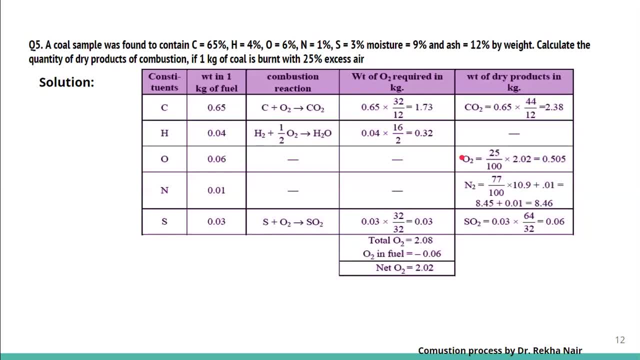 present in that 25 percent will go as flue gas. so we need to calculate that. so 25 percent of net oxygen, that is 2.02, as calculated for 100 percent, that will come out as 0.505 nitrogen. i said whatever amount of nitrogen is present in the fuel, that all nitrogen will go waste and even 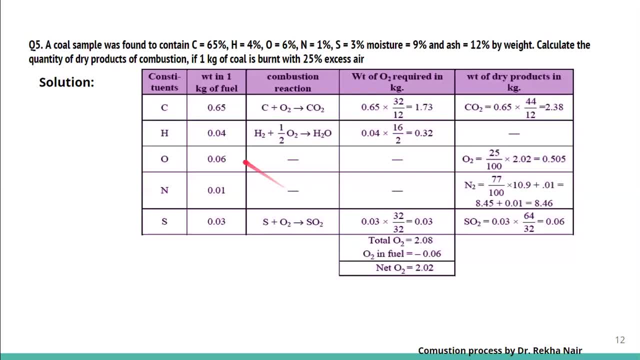 the amount of nitrogen present in the air also will go as waste. so the amount present in the fuel is 0.01, so that 0.01 will go as flue gas, and here we need to calculate 77 percent of total air. so for calculation of air we did- minimum weight of air is equal to 2.02- into 100 upon 23. 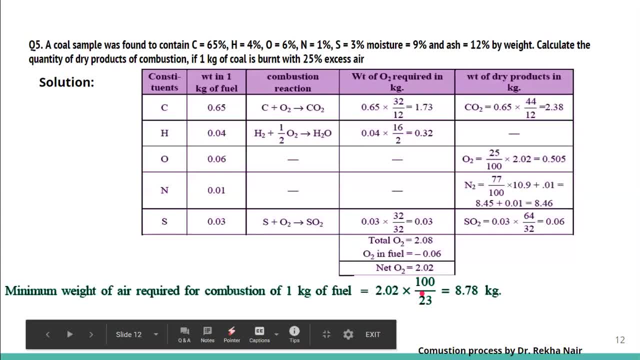 because air contains 23 percent of oxygen in terms of mass and here because 25 percent excess air is given, we need to calculate for 125 percent. so multiplied by 125 percent we have 8.78. 8.78 into 125 percent. that will come out to be: 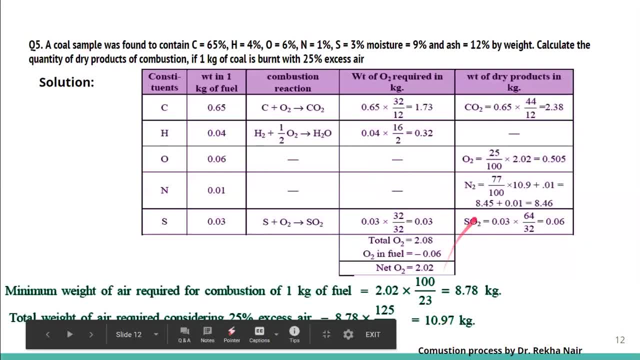 10.97. so, as i discussed in the previous numerical, also 77 percent of 10.97 we need to take if there is no excess air, we need to repeat the calculation as i explained in the previous numerical. also 77 percent of 10.97 we need to take if there is. no excess air. if there is no excess air in the fuel, we need to take at least 8.. Jorge's my scientific open. you take it 8. 00 hand microscope. if there is no excess air in the fuel, we need to take X and P seven. 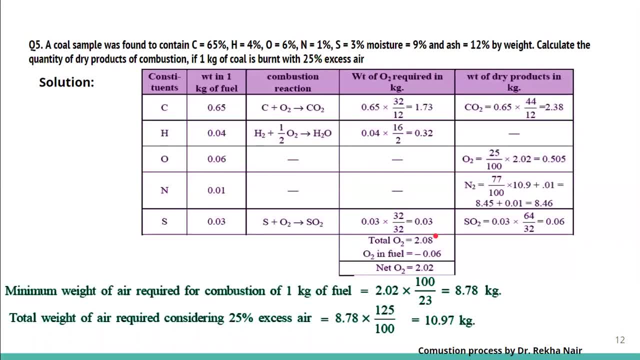 end userwał, so for calculation. so, for example, k k my original machine, where 25 percent of oxygen for 0.08 will come out to be 20.ということで, and excess air given, then we need to take only 8.78. this is, which is nothing but the minimum weight. 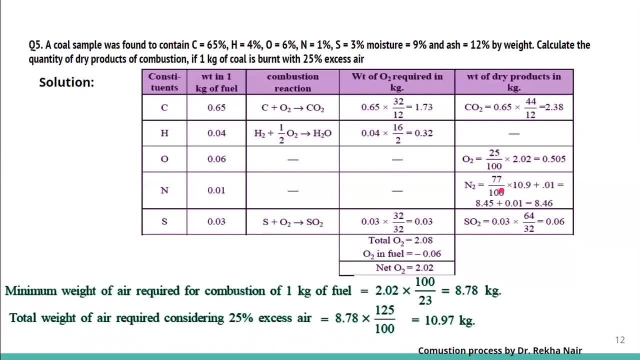 of air required. so the nitrogen will come out to be 77 percent of 10.97, plus 0.01 from the fuel given will come out to be 8.46. SO2 is equal to 0.03 multiplied by 64 by 32, because the 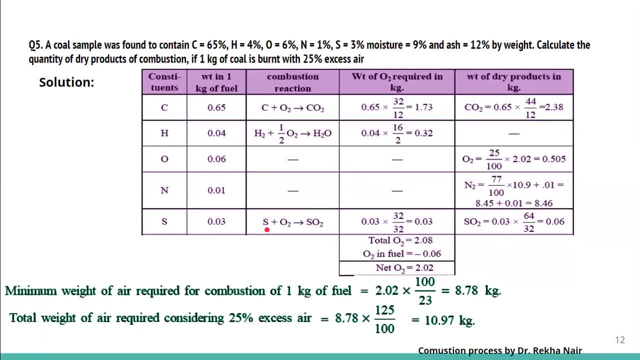 molecular mass of SO2 is 64. so 32 gram of sulfur will give 64 gram of SO2. so we are multiplying it with 64 by 32. now let us do the amount of dry product. so we need to calculate the percentage of dry products. here we have done the calculation for total weight of air. 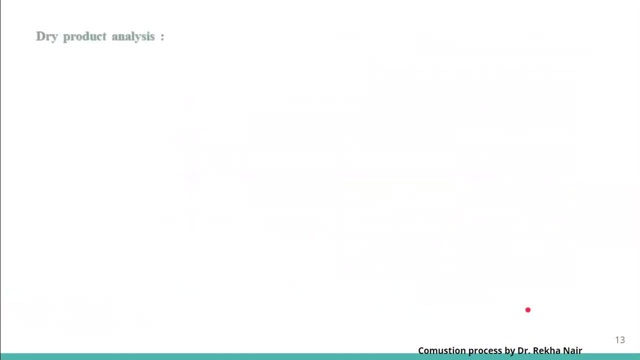 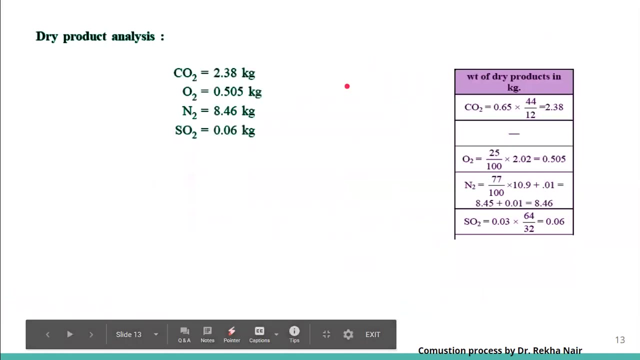 these are, these are the values that we have calculated. so we have done the calculation for total weight of air. so we have done the calculation for total weight of air. carbon dioxide: 2.38. oxygen is coming out to be 0.505. nitrogen is coming out to be 8.46. SO2 is coming out to be 0.06 kg. so total weight is equal to: we have to sum up all this: 2.38 plus 0.505, plus 8.46 plus 0.06. now for calculation of percentage of carbon dioxide, we do 2.38 divided by total weight of dry product. 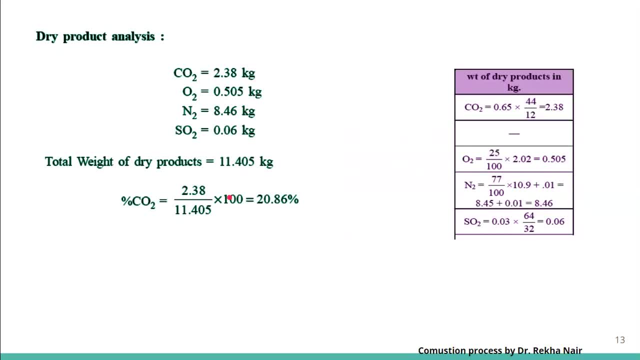 we do. 2.38 divided by the total weight of dry product is just level 9, 405 x 100. that is 20 million. 8, 6 and 4 oxygen, 505 divided by 11 and 4, 505 x 100. 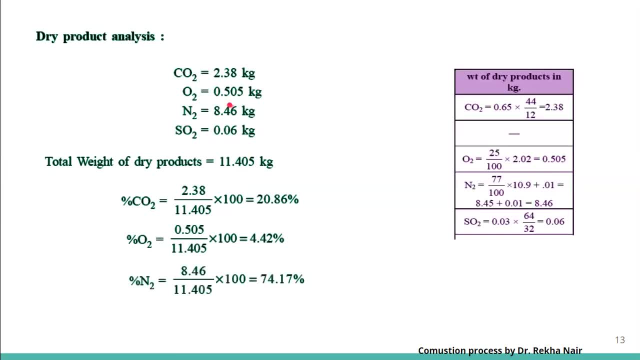 and 4 oxygen 505 divided by 11 and 4 505 x 100 and 4 oxygen 505 divided by 11 and 4 505 x 100. for example, melz, CO2 Springs and ROC Z valid by 11 곤. 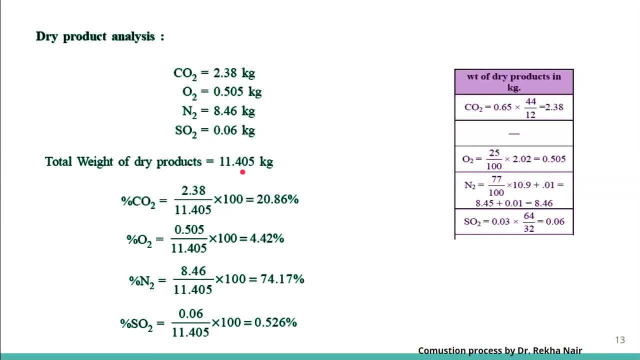 5 multiplied by 100, that is 0.5 to 6 percent. these are the percentages of dry flue gases or dry products formed in the combustion process. that's all for today. thank you all.